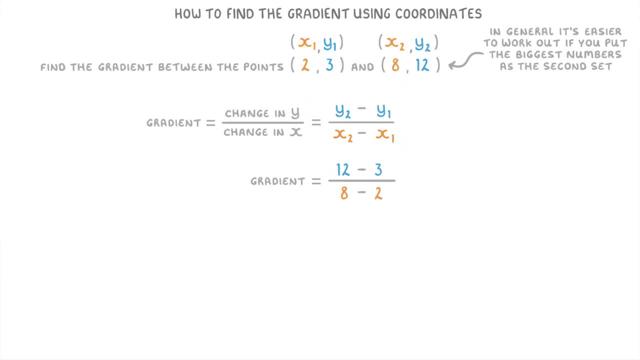 we'll have 8 minus 2 on the bottom. Then we can simplify this to get 9 divided by 6, and that would just be 1.5.. So we know that the gradient between our two points is 1.5.. 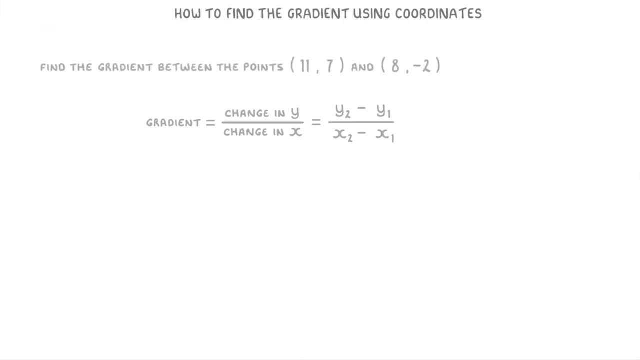 To give this some more practice, let's have a go at this one where we need to find the gradient between the points, and So the thing we need to do here is choose which pair is going to be the first coordinate and which is going to be the second, And remember, it's normally easiest if we make the bigger coordinate. 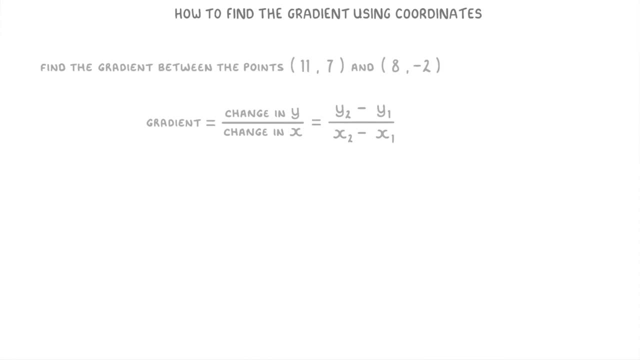 the second one. So we'll make 11: 7, the second meaning that 11 is x2 and 7 is y2.. So 8 is x1 and negative 2 is y1. Then all we have to do is plug these numbers into our formula. 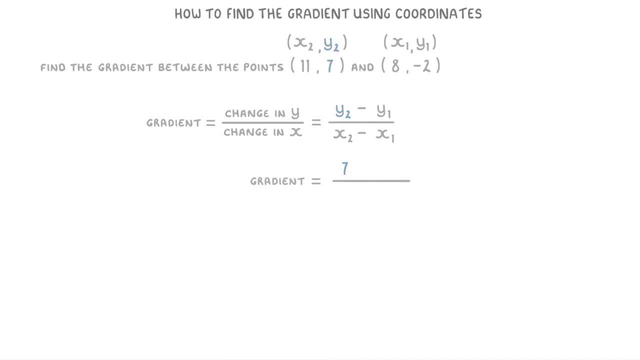 So on the top we'll have 7 minus negative 2, and for the bottom we'll have 11 minus 8, which simplifies to 9 over 3, which is just 3.. So the gradient between our two points is 3.. 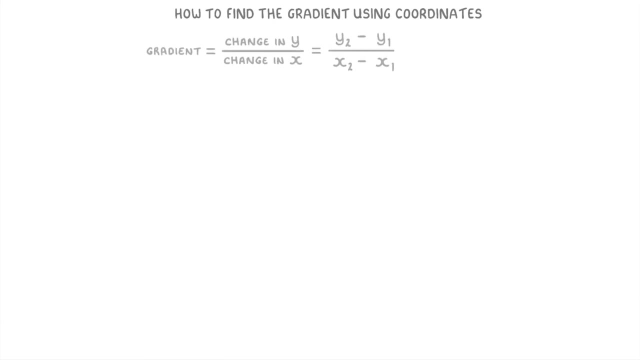 One last thing that I want to point out is that we can also use this method even if we are given a graph, because we can just pick two points and then we can simply pick the two points. So we can just pick two points and then we can simply pick the two points, and then we can simply pick the two points. 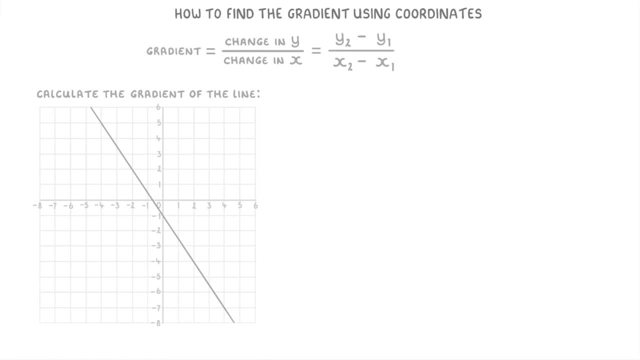 So for this question, where we need to calculate the gradient of the line, we'd start by picking any two points along the line like these two, and then label them both, So 0, negative 1 and 4, negative 7.. Next we need to choose which one's going to be the first. 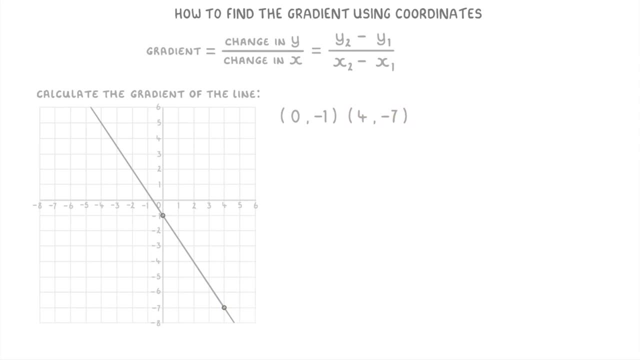 coordinate and which one's going to be the second. But it doesn't really matter this time, because this one has the bigger x value, but this one has the bigger y value. So we'll just pick this one to be our first and this one to be our second, And now that we know what all the values are, we just plug. 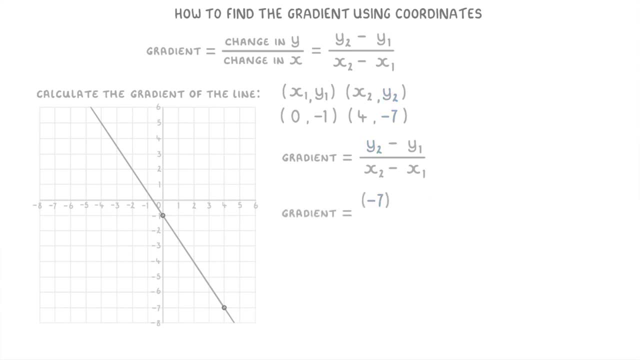 them into our formula. So negative 7 minus negative, 1 over 4 minus 0, giving you negative 6 on top and 4 on the bottom. So you just do negative 6 divided by 4. Which is negative 1.5.. And that's your answer.